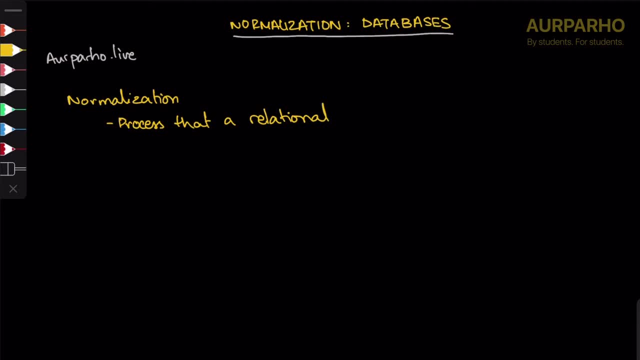 is improved. I'll write it down. The process that a relational database goes through, goes through or structured. in the end- sorry, in the end- it is structured such that data integrity improves, data integrity improves and data redundancy is minimized. Data redundancy: 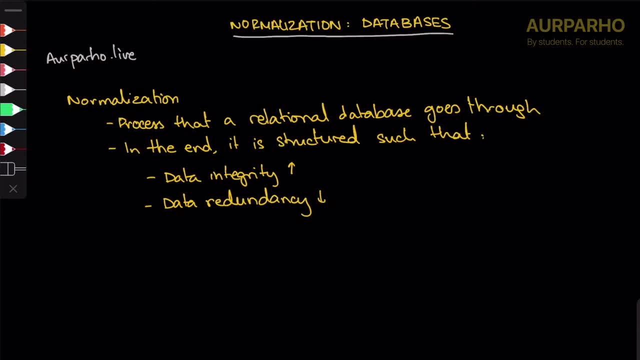 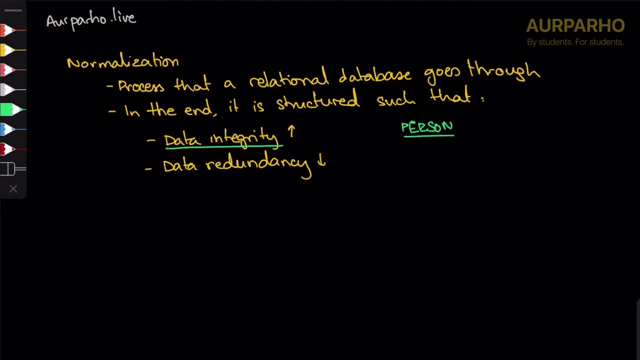 is minimized In the terms of data. integrity basically means how accurate and how consistent your data is throughout database, like, for example, if I say that I have a person's table, it's called person and it has his name, his birthday, date of birth and his age height. now, if 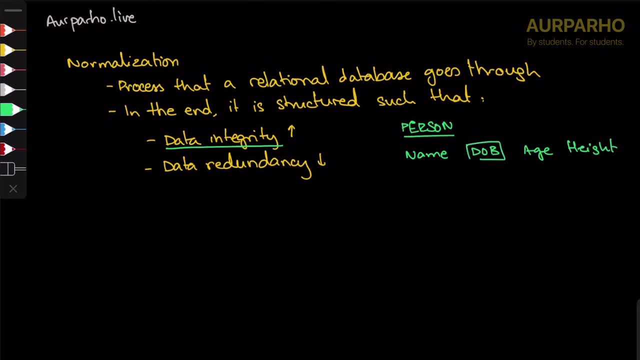 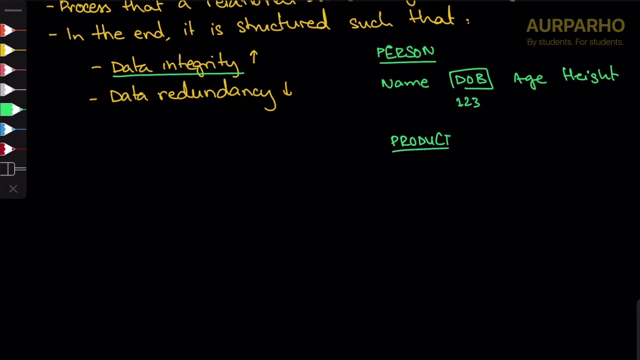 date of birth has any random number other than date- just one, two, three- and it doesn't follow a format. it's not a date that that means my data is my data. I don't have a good data integrity. similarly, other mere basic relation, other mere buzz: do Saturday village is gonna have product or it's my product ID? 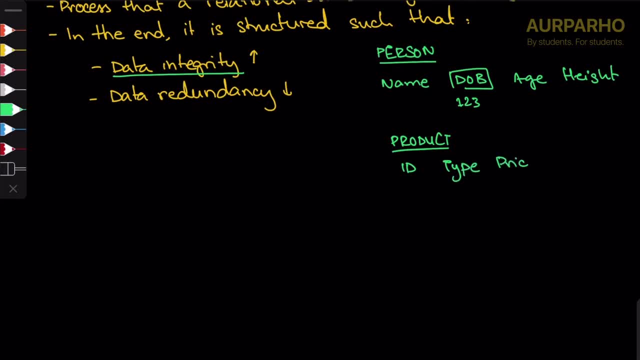 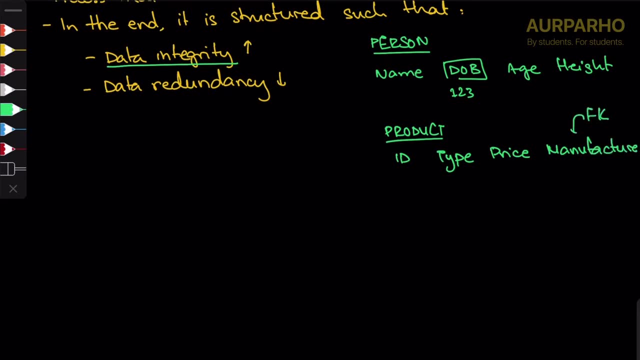 hair type price, or a male bus, a column, a manufacturer or manufacturer year- foreign Kia is Kamala business. manufacturer IDs only which link to and other manufacturer table. so yeah, up whoa do. what if I have an ID that's not present here, or, for example, this ID: 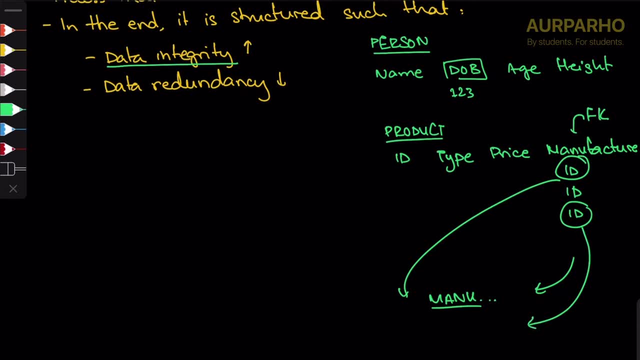 is not present here. that means, again, I don't have good data integrity because I am referring to something which is not present: my love, my bull, long cable or a hierarchy. well, if you move on, a little key with a star database, essentially toot-jata. so, yeah, it's referring to something which is non-existent, it's. 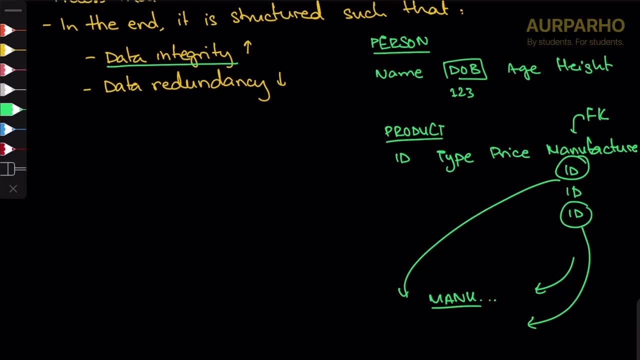 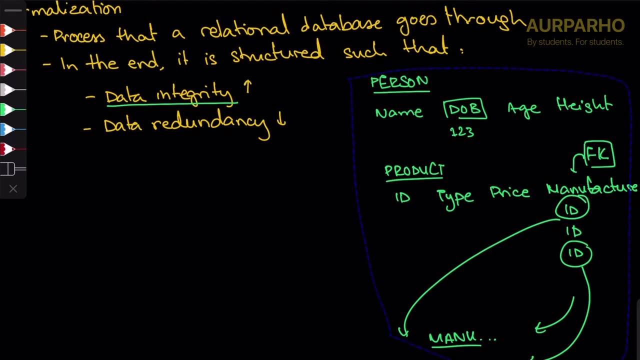 gonna return an error when you try to. you know query for that. so it's Lea. yeah, this specific type which I mentioned about the foreign key, that's called referential integrity and it's part of data integrity. so, in general, data integrity is how consistent and accurate your data is. what about data in? 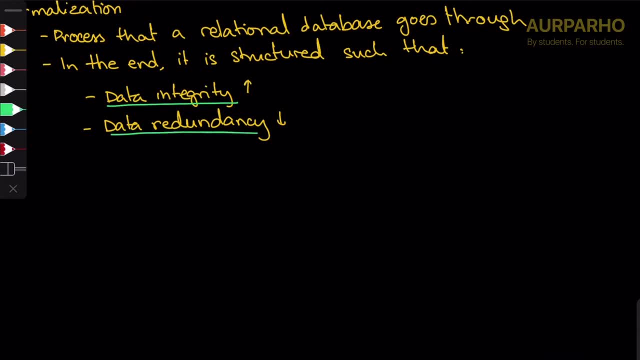 redundancy data. redundancy is the degree or the number of times your the same data is stored in the same database. so like, for example, if I have the same again, we'll go with a person. let's go with a person example again, and let's say we're storing the information about a person called John. 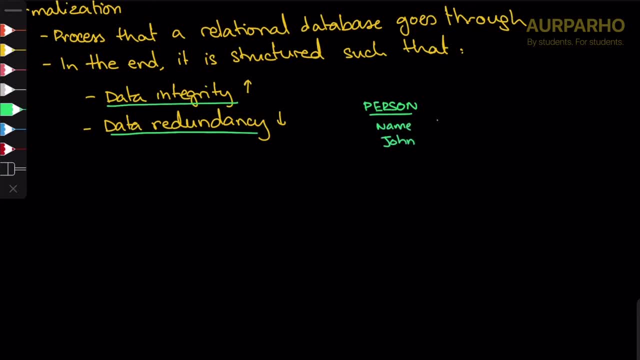 so his name is John, his DOB is, let's say, oh, 212, so 2nd December 2000, and his age would be 20, 20 years old, I think. so let's say: this is the information that we're storing. so if we are storing this in the person database, and then let's say we 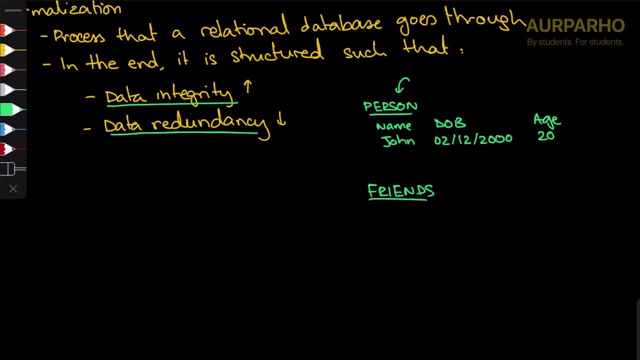 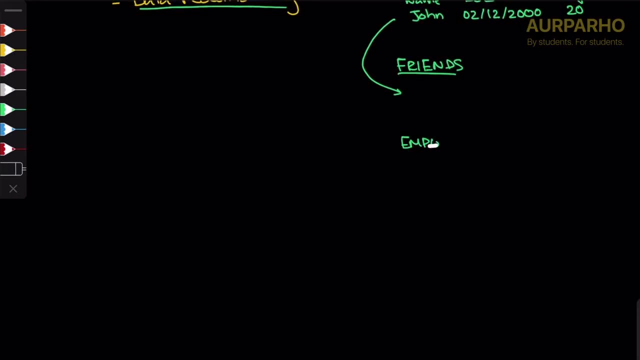 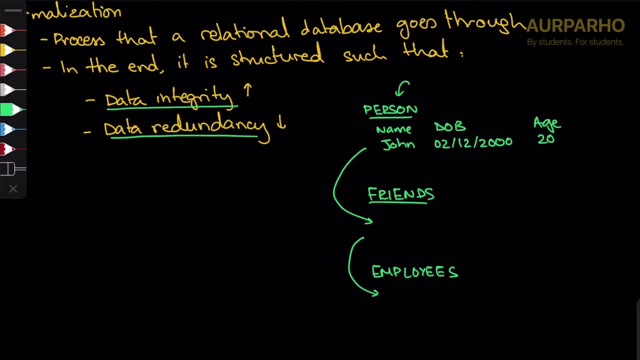 store it in the friends database- again this, this same, this same information- and then we store it in the employees table- again this same information. and let's just say this is a database that requires these three tables somehow. so we store this exact information three times, which is a waste of space, because we could refer to it at one spot and then only. 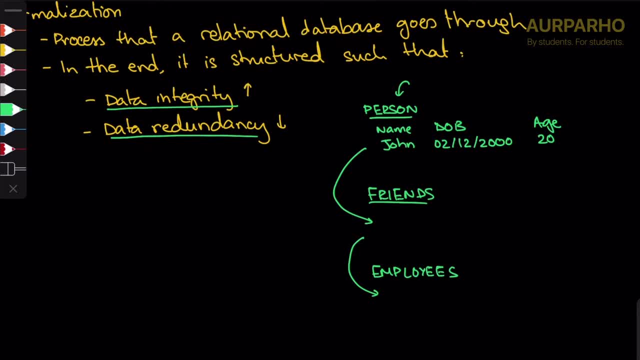 store it one, so it has more data redundancy. so when we build a relational database, a good, a well structured relational database has minimal data redundancy because you have to maximize the storage. it means you have to minimize the amount of storage each record or each data item is taking. so if you store it three times then it's going to take a long time. 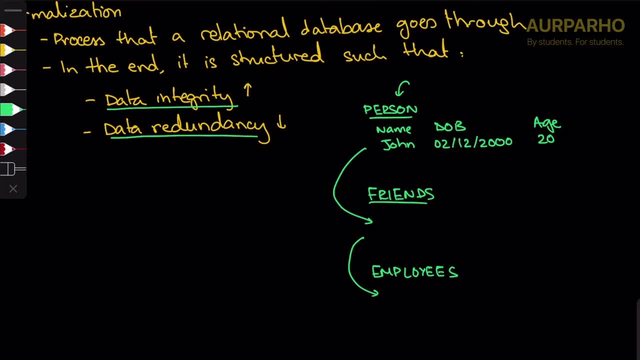 triple the storage it would normally take. that is one reason. or the second reason is that if I, for example, update its date of birth, suppose we entered it in error and it's not 2000, it's 1999, so I have changed it here. but since it has been stored in multiple places, 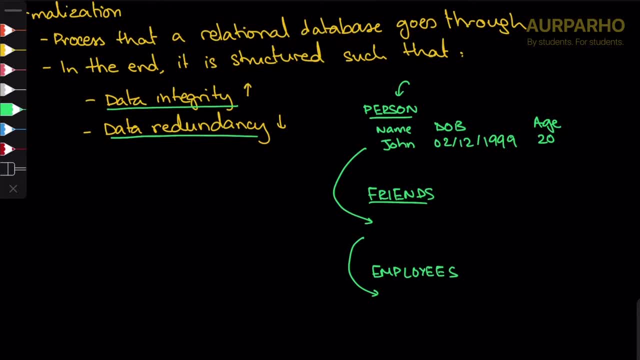 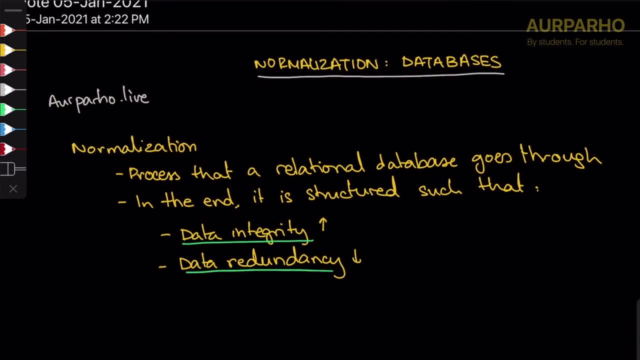 we have to update it multiple times throughout the database, and sometimes we might not be able to do that and there might be some records which show old, inconsistent data, so that is also not good. so yeah, so that is all to say that when we normalize a database, we improve it by improving. 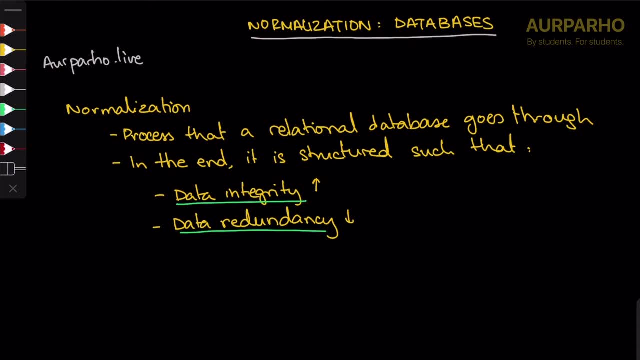 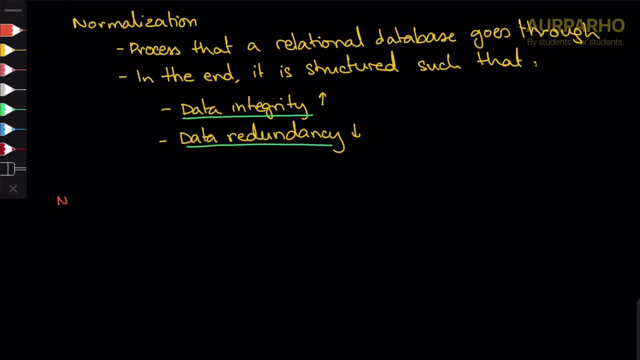 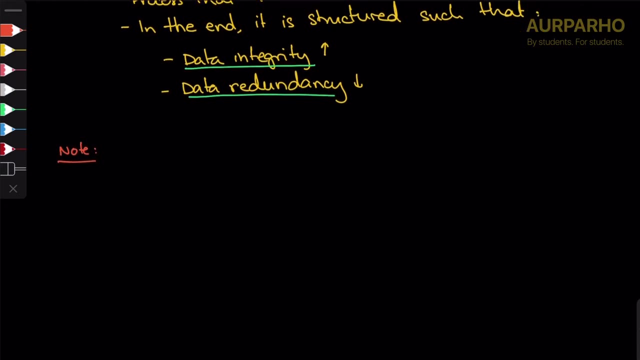 its data integrity and minimizing its data redundancy. so now let's begin. oh, also a note, a side note, and it's also written in the note: all normal forms are progressive. what does this mean? this means that if a database is in 3nf, so which means third normal form, third normal form if a database is in 3nf, it means 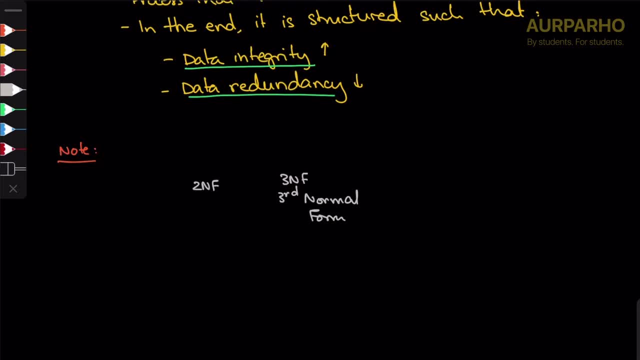 that it is. it was first in 2nf and before that it was in 1nf, so you cannot be 3nf without being in the second and first normal form. so that's what it means to be progressive. okay, so let's actually begin with the normalization process. 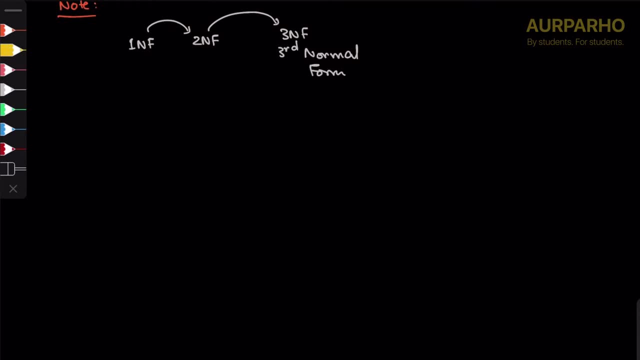 the first step in this process is the first normal form. the first normal form, first normal form attribute only has atomic data. atomic data, so you know how atoms are the smallest building blocks of matter. we study that in basic sciences. so atomic data means data in which each data item is the simplest as and most single form of the data being represented. 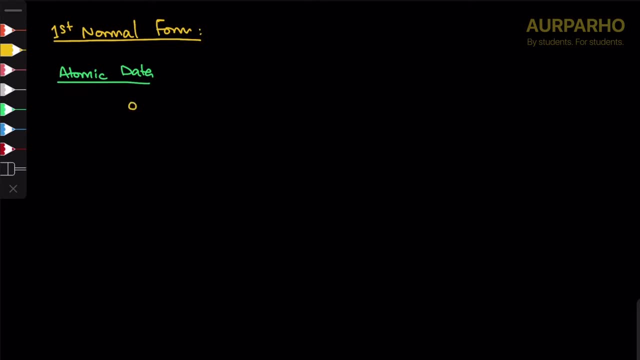 now, what is the example of this? so yeah, for example, i have an order, i have an order column. let's say we have a shop table and i have other fields, and then i have an order column. now, what do i store in the order column? i store 35 candy bar. 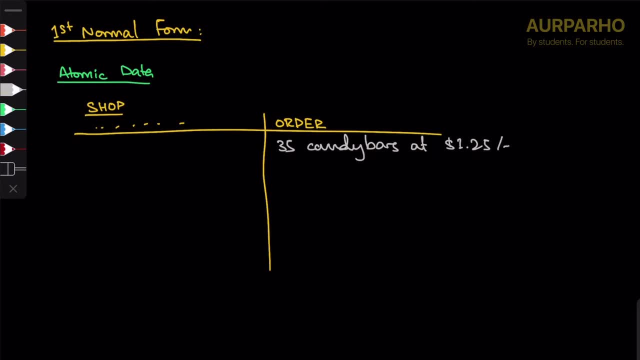 at 1.25 each means that someone has ordered. this is what the order is. someone's ordered 35 candy bars at 1.25 dollars per candy bar. this is not in the first nf, as in this entire piece of data which is in the order column, it is not atomic. it is not atomic why? because 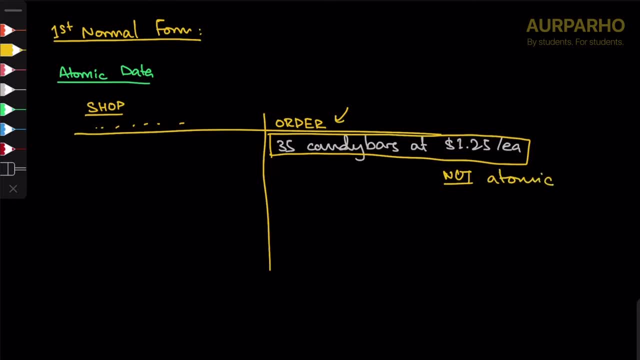 in this first nf there's actually three simpler looking bars and if you look in the order column it's not atomic. it's not atomic why? because in this first nf there's actually three simpler data types that we can split. sorry data items. it has 35, which is the quantity of the order. 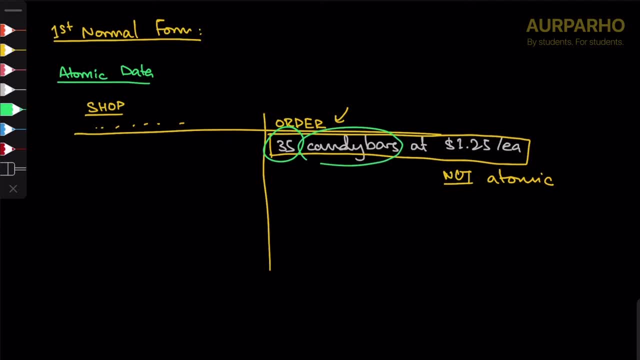 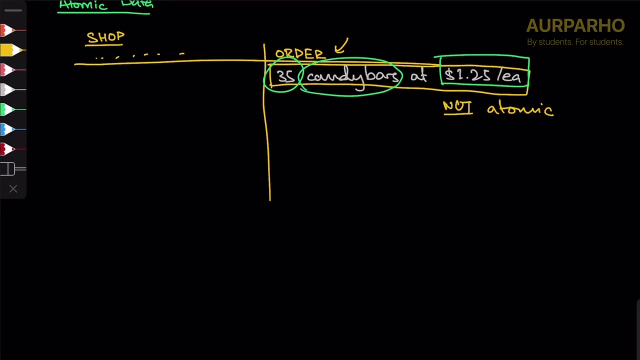 how many items have been ordered. it has product- which type of product did the customer order- and it has rate- the price per product, per unit of the product. so it has three data items grouped into one data item: time. Jabez could split career. when we split this, we will write or we will write. 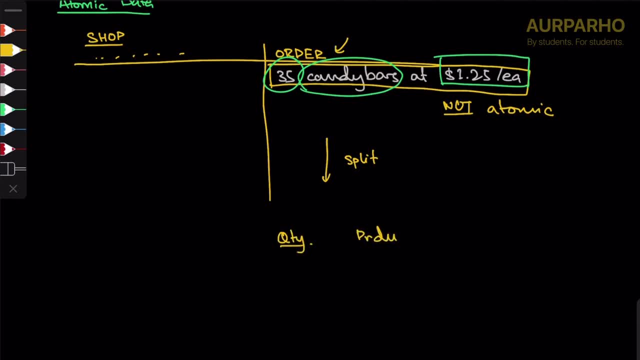 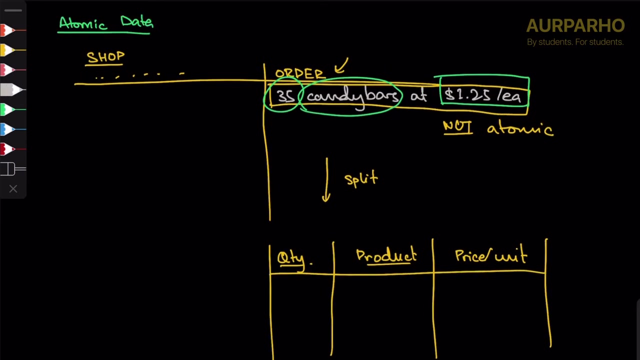 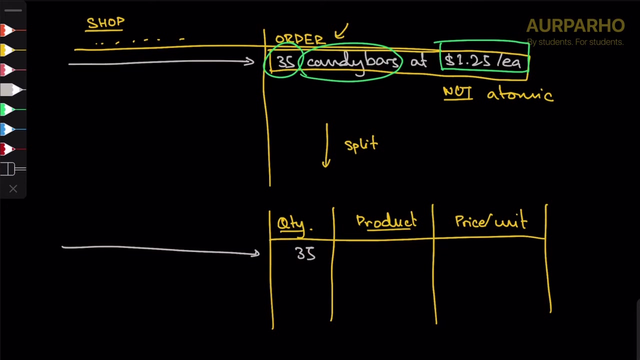 quantity, you write product, product and price per unit. if in columns on in the database, the shop database, say yeah, so this will be then splitting into, let's say the. for the same, for the same person that ordered this, if we, he would now be represented. the same data would not be represented as 35 can't 35. 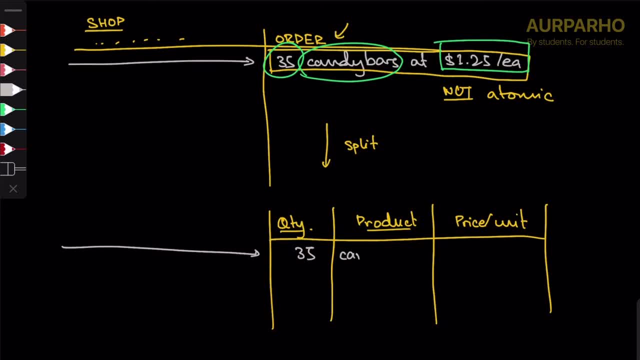 units, units of what units of candy bars and what is the price per unit? the price per unit is dollar 1.25, so this is how you would split this into this. that's one part of the first of converting a database into the first normal form, the 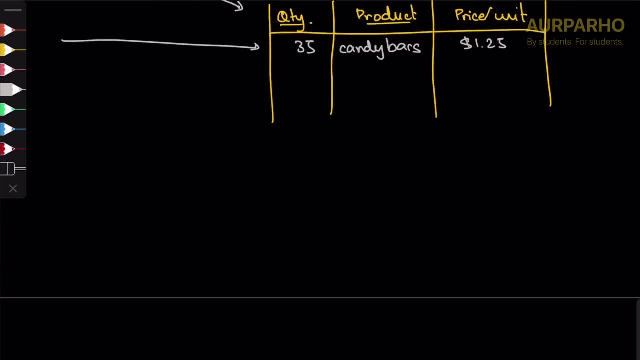 second part mentioned in the notes is each table has a unique identifier called a primary key. now, okay for that. let's say we have the same shop table and in the shop table when a customer order something, we store his first name and his last name. now the reason this is not in first: 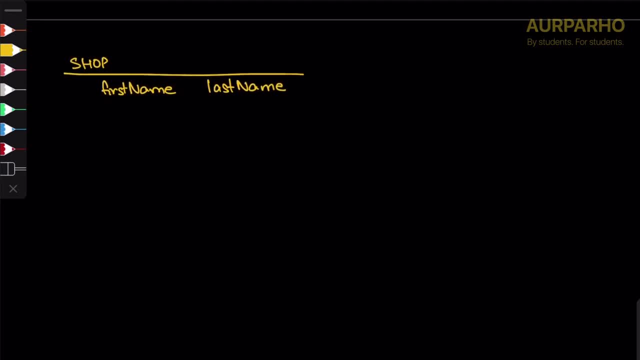 normal form is because the first name is not in the first normal form and the form is because it is possible for the for different people with different orders to have the same first name and last name. so what you need is you need a primary key. what is a primary key? a primary key is a type of attribute, so it 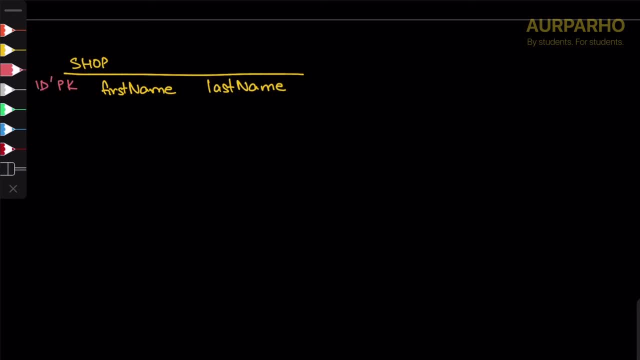 will be a column. a primary key, usually called an ID, would be a column here and it would basically be unique for every single entry in this database or in this table. at least say yeah, so, and then you want to have a primary key, and then you won't have to worry about first name and last name, the chance of first name and 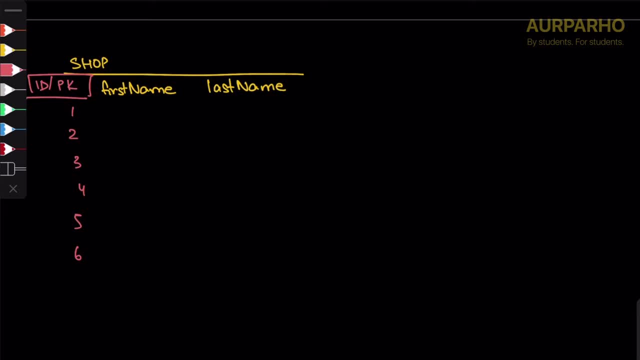 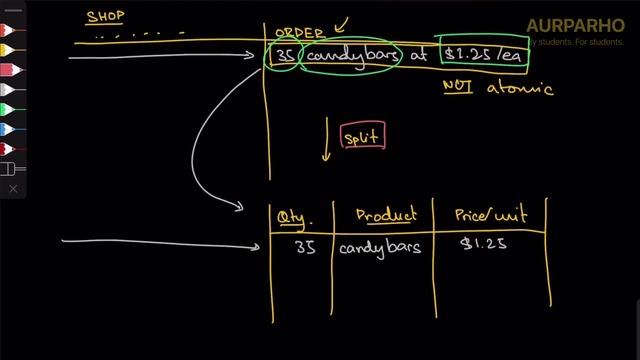 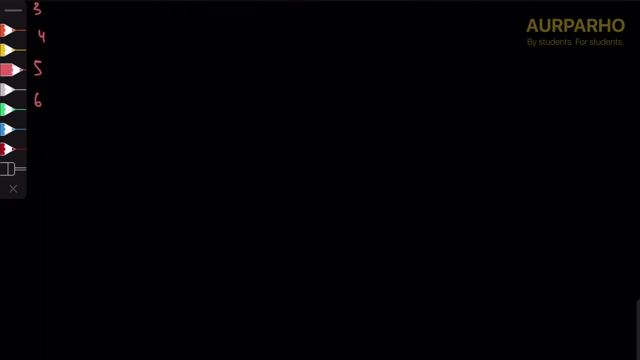 last name being the same for different people say so when we do that, when we add a primary key and when we split a group of like non atomic data into atomic data, then we can convert to first normal form. so I'll actually do that right now. I. 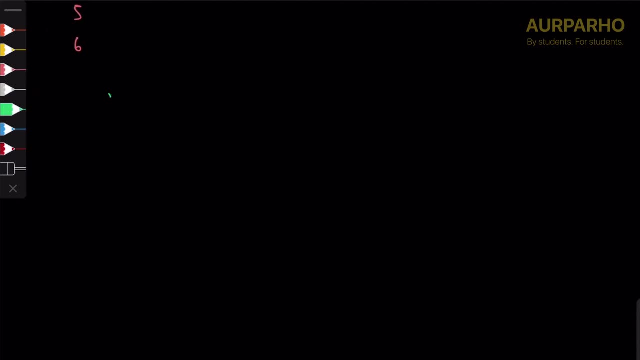 will make a sample database. let's see that's. it's called it first, normal form: first name. these are the columns: first name, last name, date order, and I'm actually just copying this from the note. um, this example is given in the notes, so I'll do. John John Smith, John Doe Brenda. 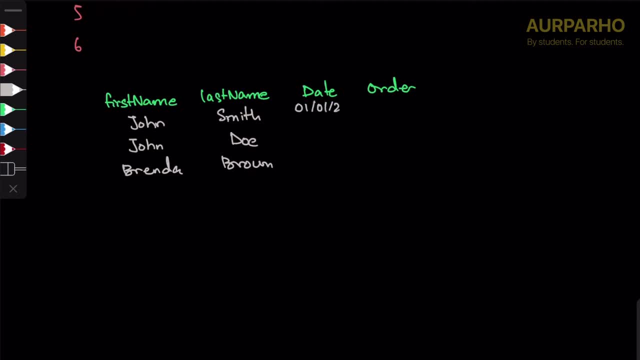 Brown, um. 010120-020319-05-04.18. should move that a bit here and yup, the order is 35 candy bars at 125 dollars per candy bar, 40 shovels at 50 each and 10 TVs at 950 each. when we convert this to first normal form. 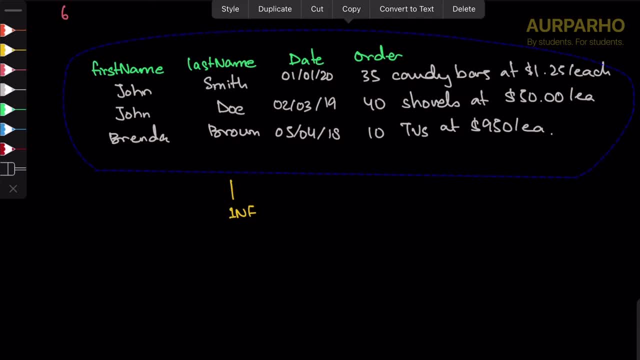 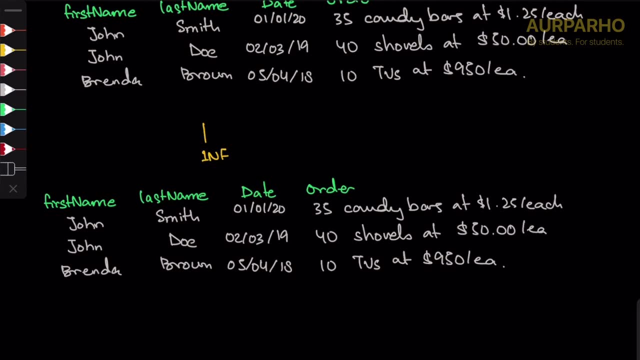 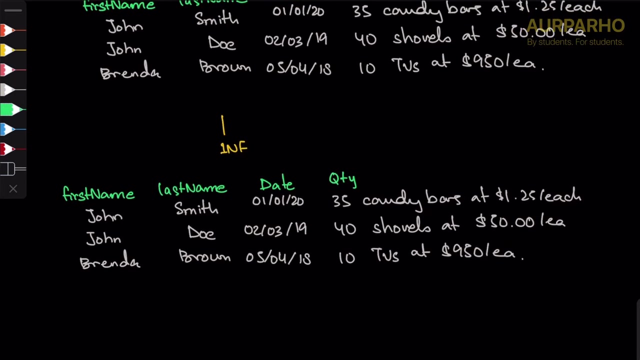 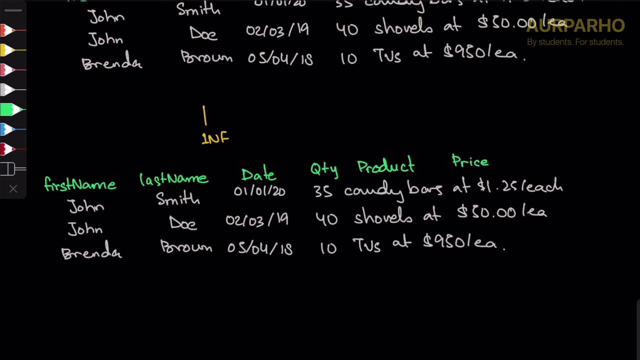 let's copy it. when we convert this to first normal form, we split the order table, the order table into multiple, multiple columns, multiple fields, and we will call them quantity. let's erase this. well, no, let's call them quantity. we'll call this product and we'll call this price per unit. so now there are three. 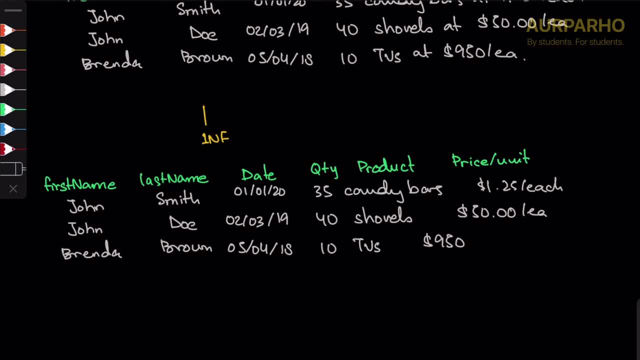 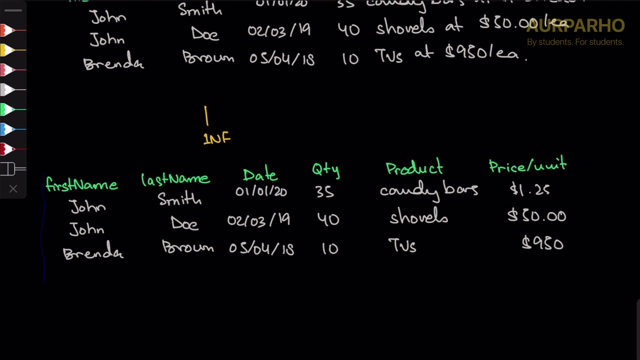 columns and we can erase this, we can erase this and we can rearrange everything else so that becomes: that comes under the product field and this comes under the price per unit, and I'll space it out better so it's clear. and this, oh also, before we have to add the 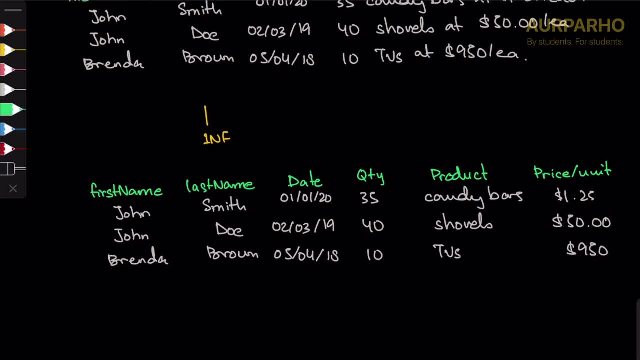 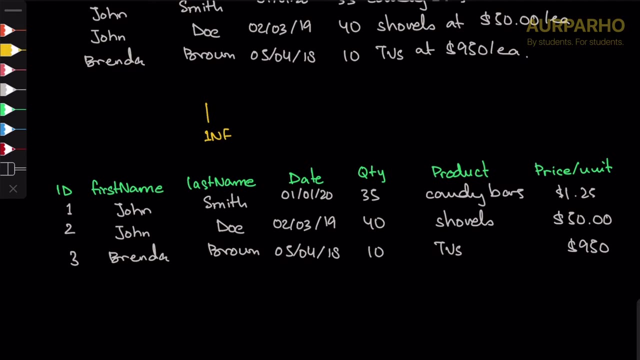 primary key, the ID. so we'll add that now and we'll add an ID, a simple ID. you will do one, two, three and we'll call this. well, let's just call it ID for now. so now this is one NF, this is a database that has been normalized to the first normal form. so 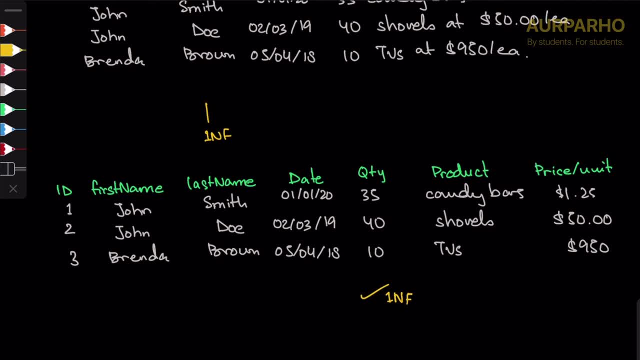 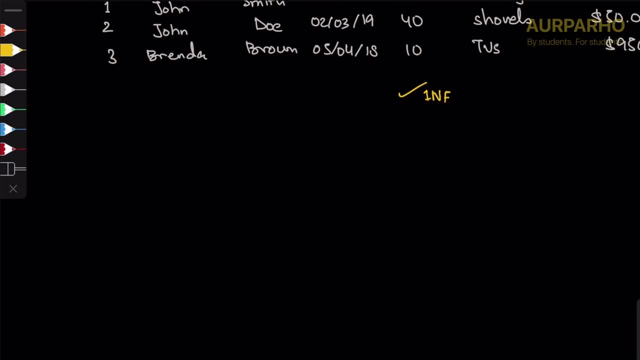 the group of. we broke up the group of attributes and we added a primary key. now the second normal form. the note says every non prime attribute depends only and only on the primary key, plus there are no partial dependencies. okay, now let's move on to the second normal form, 2NF, the second normal form. 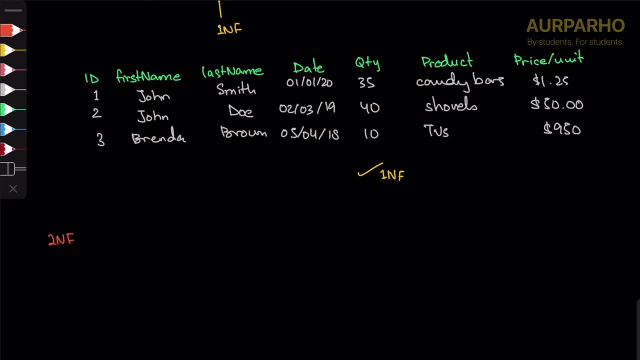 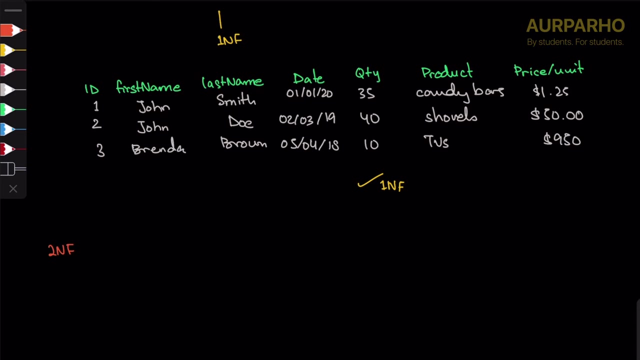 states that every non-prime attribute depends only and only on the primary key. there are no partial dependencies. essentially, boiling it down to the most basic language, which means that a table should represent data about one entity. so yeah, if we look at our first normal form, the first normal form table, it's not in 2NF. 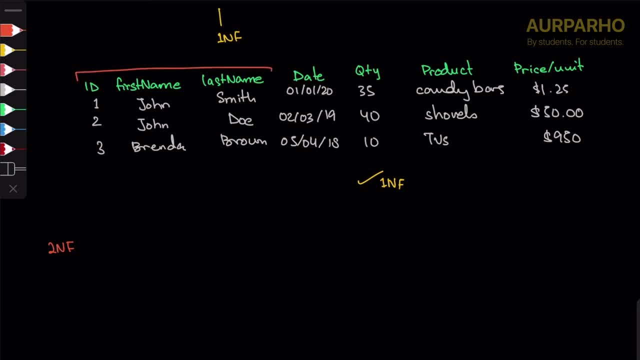 because we don't know if it's representing data about the customer or the order or the product- yeah, order and the product that was ordered. so there are like three entities that we're talking about in one table and that is not in second. normal form and, as a rule of thumb, it's telling information about: 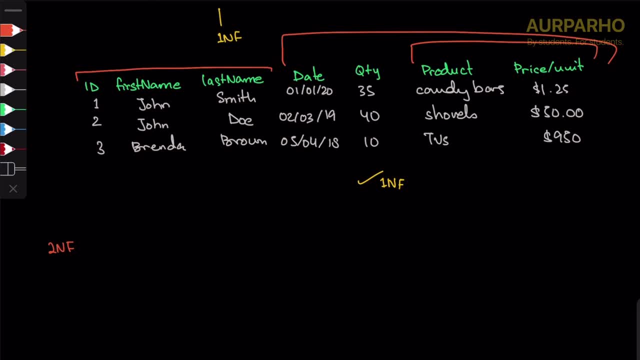 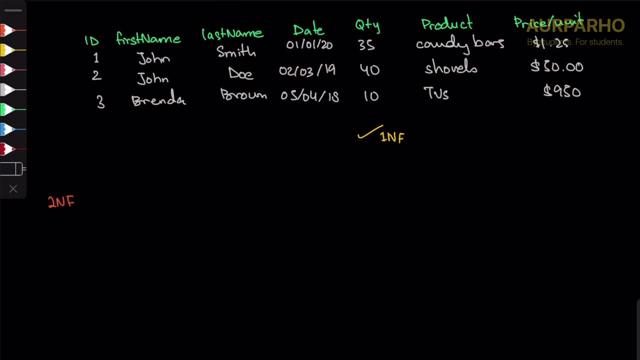 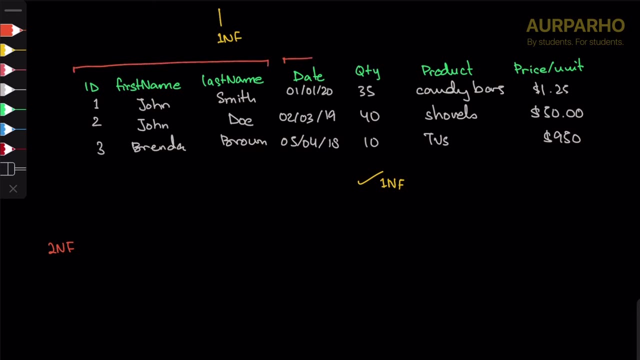 one entity and a second entity and a third entity. that means that that table is not normalized and you need to normalize it. so let's normalize this to second NF. now we know we can see that they're primary, primarily two groups. we can talk about the customer details and we can talk about the order details. so 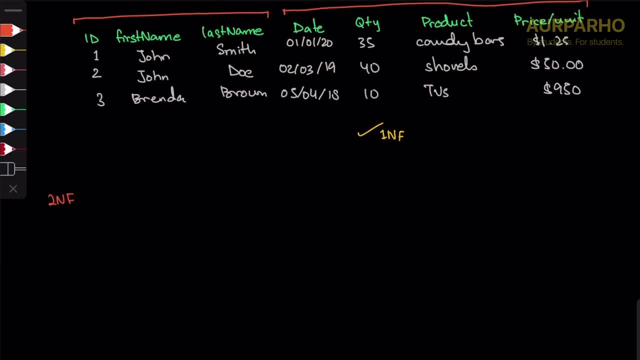 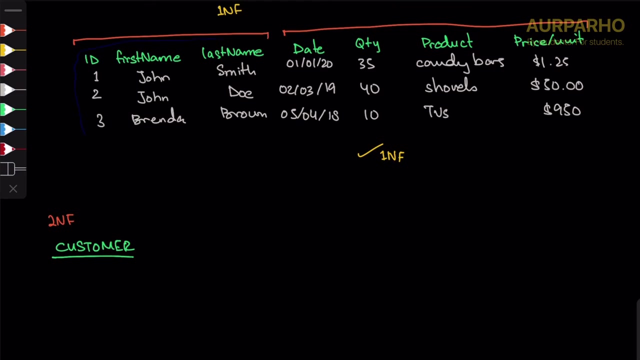 let's let's split this up into two tables. let's say, let's call it the, let's call this the customer table, and in which we'll have ID. well, I'll just copy it so I don't have to waste time rewriting all of this. we will have all of this. in fact, we will rename the customer, the ID to. 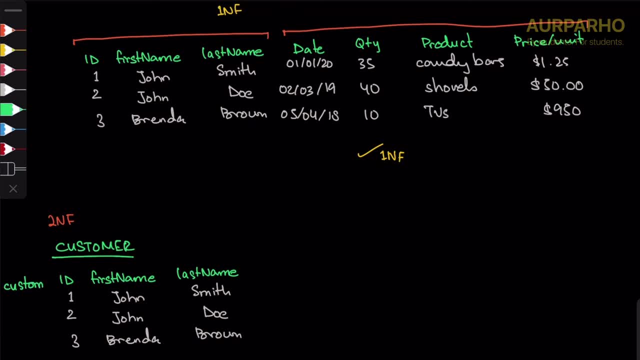 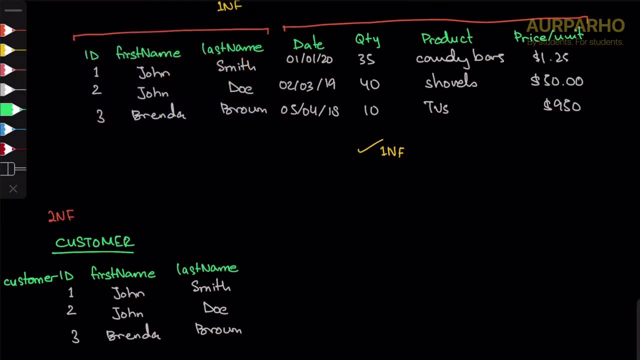 customer ID, because now we're gonna have, we're gonna start having- multiple ID. so when you keep track of which ID is which, so that this is a customer table and we can have a second table that we'll call orders, the orders table, and in here we 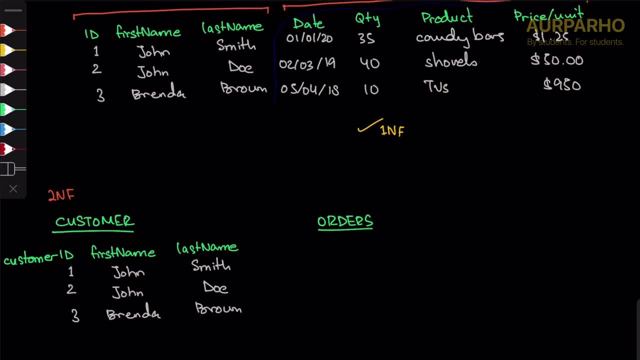 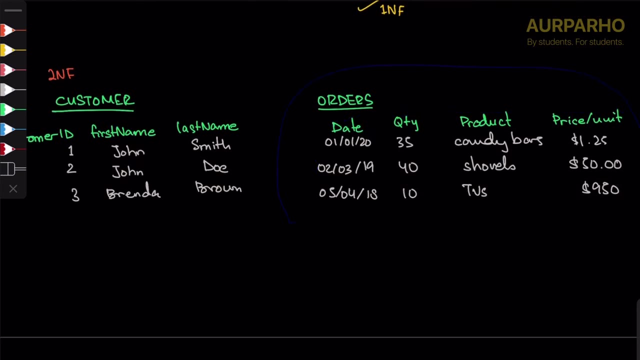 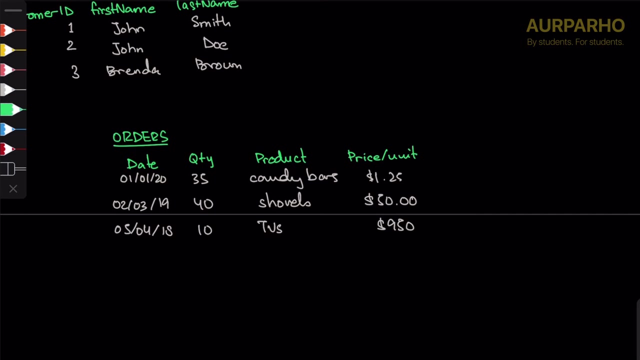 can copy all of these details and remember we need to have a primary key worship. you can copy all of these and here, actually, I'll move it down below. so, yeah, and we need an orders id. so we need orders id and let's just go with one, two, three and we also. 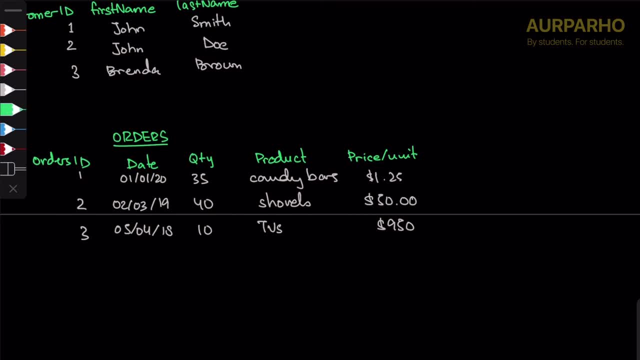 need to refer to which customer is actually ordering this certain order, for example, like which customer is ordering 35 candy bars at 125 candy bar each on this date, and for that we need to include the customer id, and here the customer id is going to be a foreign key. 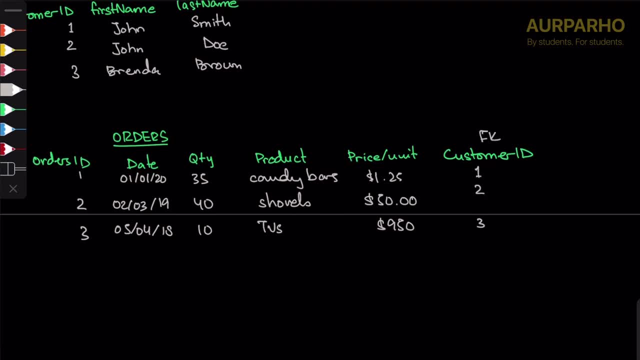 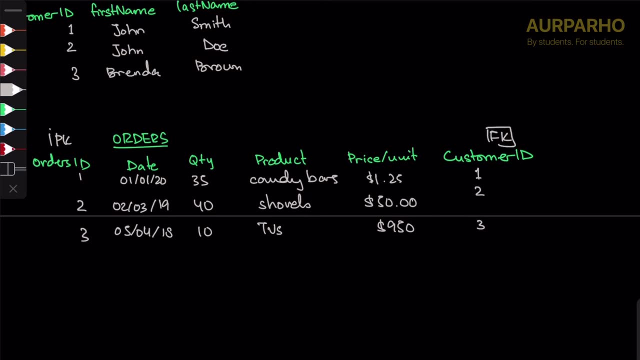 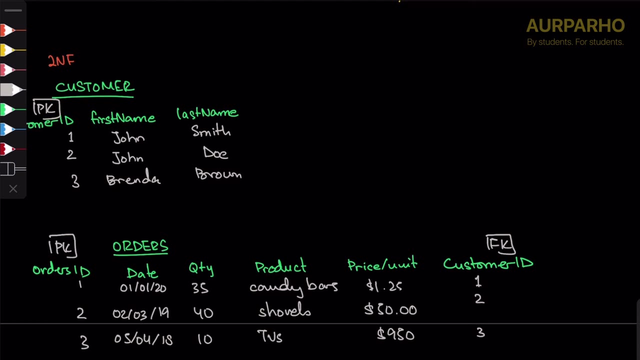 and this is going to be a foreign key, and here, just to point it out, our primary key is orders id. here and here, this is our primary key, see, and that is that now we have normalized our relational database into the second normal form. so let's go ahead and do that, and let's go ahead and do that, and let's go ahead and do that. 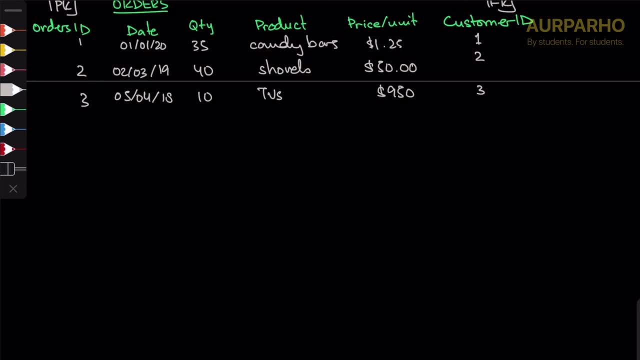 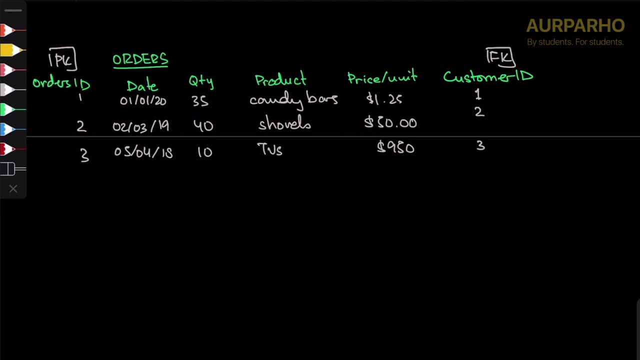 moving on to the third normal form, attributes are determined only by the primary key, the one we just converted into the second normal form. if you look at this particular field, does this change necessarily as the orders id changes? let's say, for example, we have a next person orders, so order id number four: order is a certain something: zero, seven, zero. 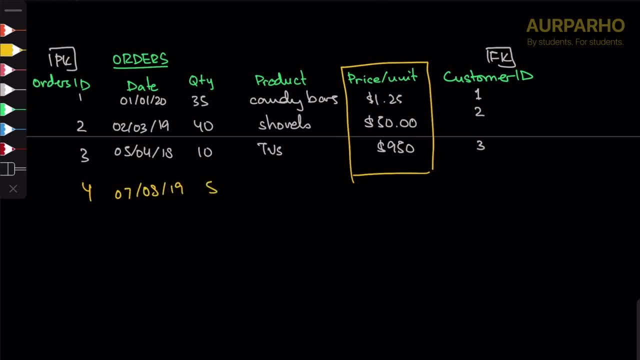 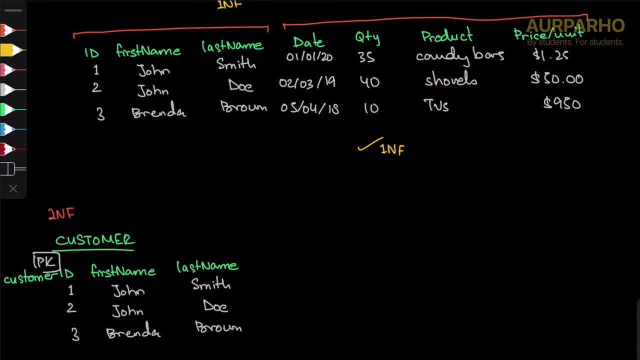 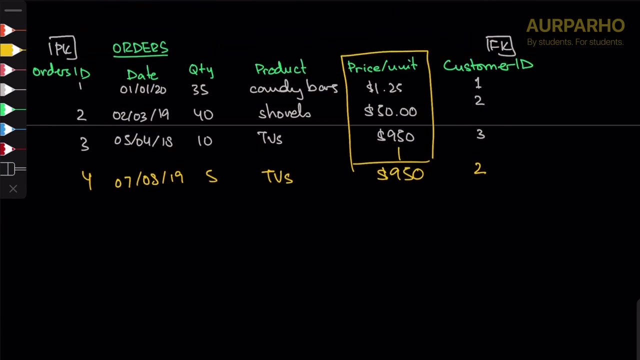 eight, nineteen, whatever, on that date he orders five um, five tvs at 9: 50 each, because tvs are priced at 9: 50 per tv. and this is customer number two. for example, john doe. john doe order, that's his order, um. so you can see that from the order. id changed, so the primary key changed, but this: 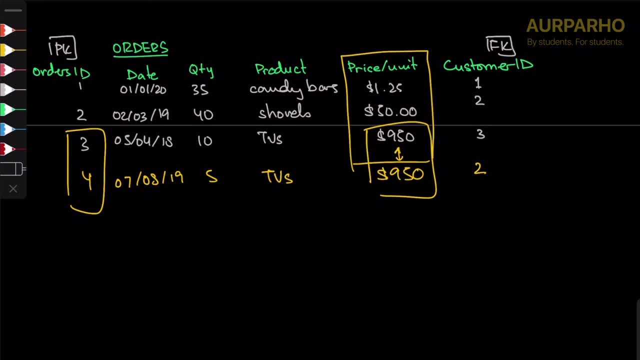 did not change. that means this does not necessarily vary. it does not necessarily change as the order id changes, and so we can see there's a partial dependency here. we can see that price per unit depends more on the product. so it depends what the product is on the actual order id, so that 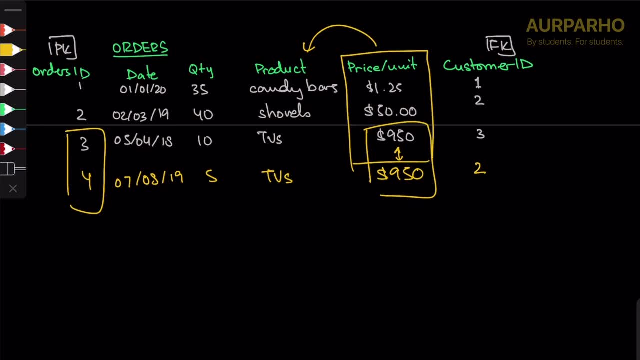 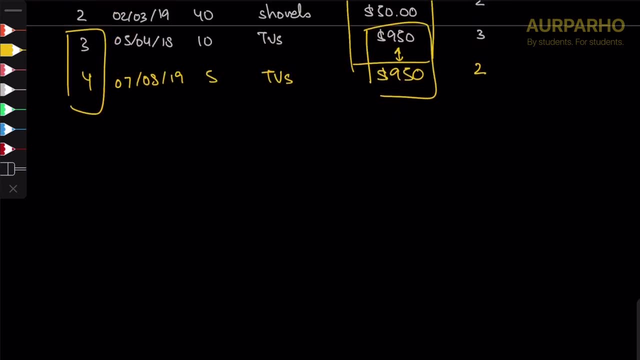 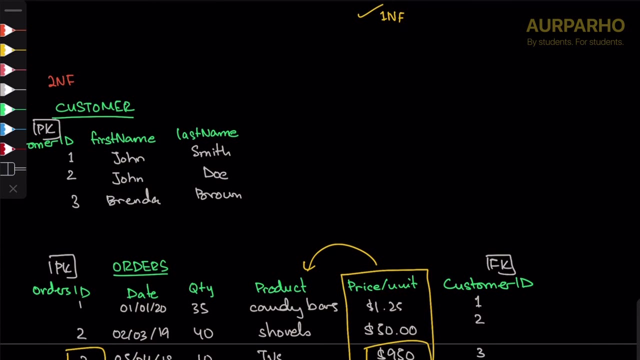 indicates. that suggests that we can further break this table down, we can further split it, so it is more succinct, right, so to do that. we will convert this into third normal form and the the customer thing, the customer table doesn't. the customer table remains unchanged. the customer table remains unchanged. so i'll just copy that down here. 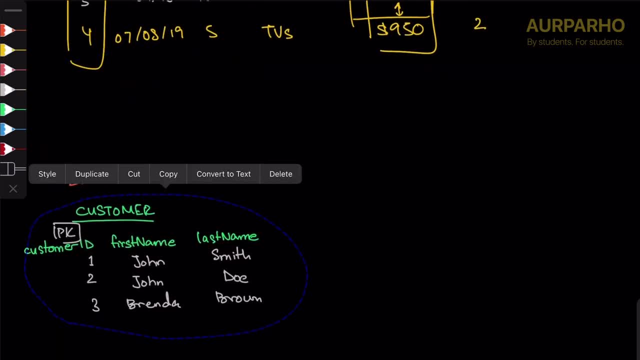 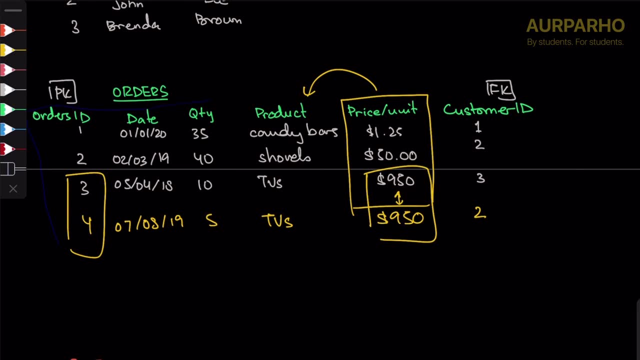 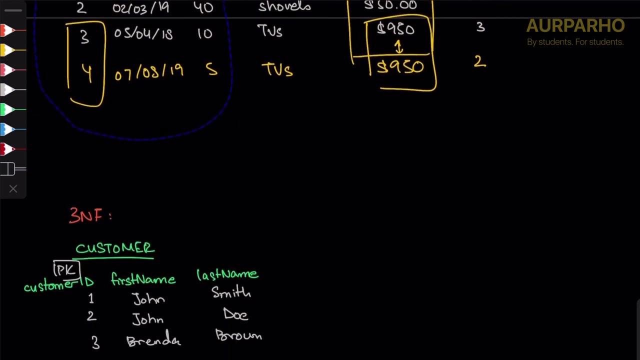 and that's the customer table. the orders table, however, is gonna be altered so we can see: we need the orders id, we need the date of the order, we need the quantity, can copy that, and I'm gonna remove this just so that we can maintain the same. 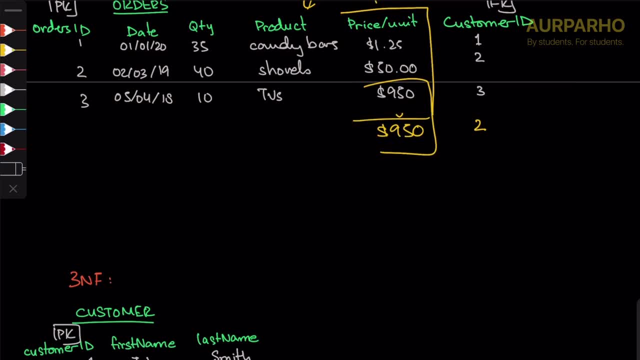 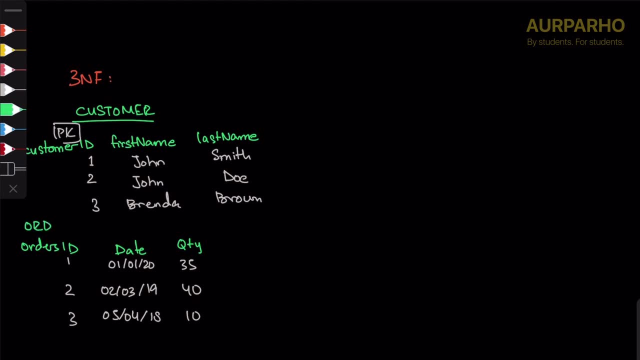 data set that we had going into this lecture. okay, now we have the orders table- let's call this orders- and not only will we add, will we keep the customer ID so we know who is ordering what. now we'll add a product ID as well, so that we know what are they ordering, because we split the products into a 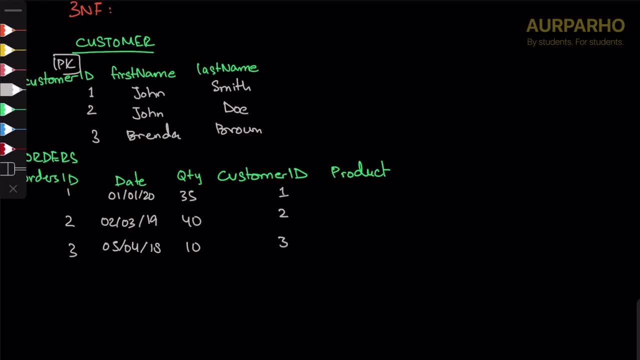 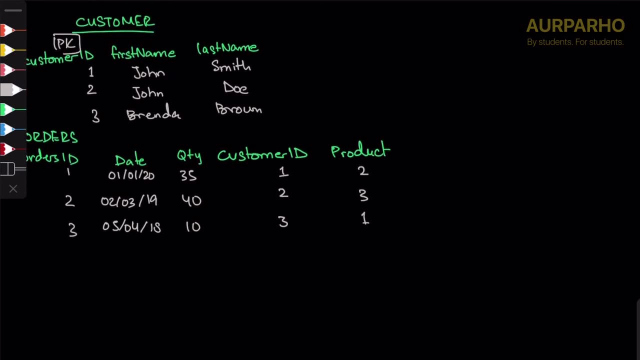 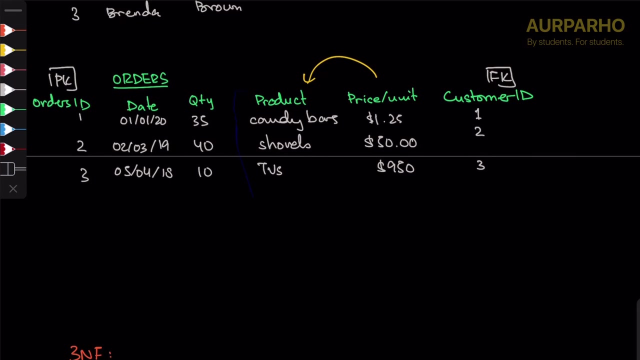 second table. so this was one, two, three. let's call this two, three, one and we will arrange our product table accordingly. I just wanted to vary the one, two, three, so it doesn't always seem like it's always gonna be one, two, three. so product price unit, customer ID: we were gonna leave customer ID out of it.